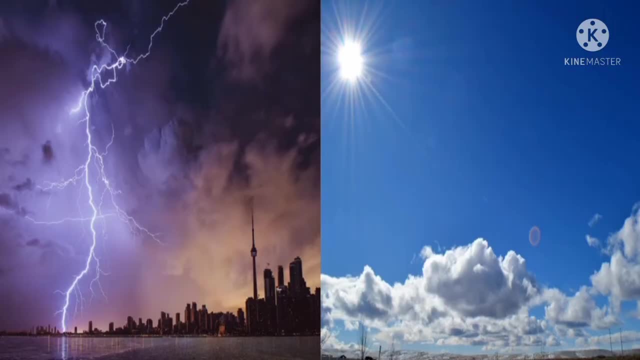 variable x. Similarly, friends, every day the weather keeps changing with respect to time. Also, if it is sunny at one place, then there will be thunder or lightning at another place. So this way, the weather also changes with respect to time Or with respect to the place, And it's a common sight to see the petrol level change as the usage. 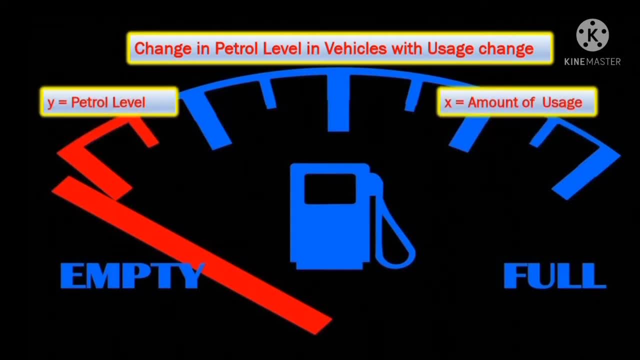 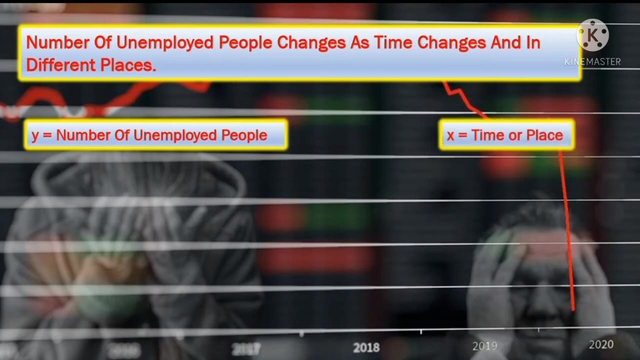 of the vehicle increases or decreases. So here you have y as the petrol level, friends, and x is the amount of usage, And friends. what about unemployment? Well, that too changes with time, Maybe every month or year, and it also changes from place to place, And stock markets are no different. 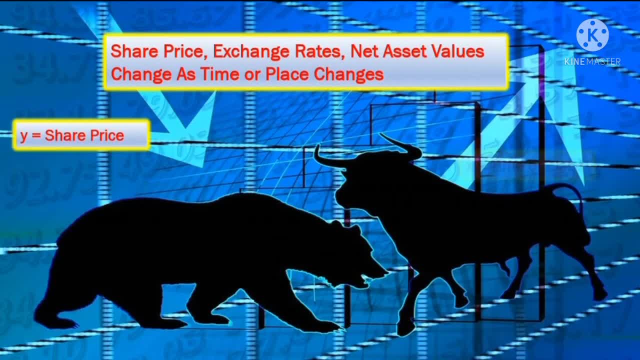 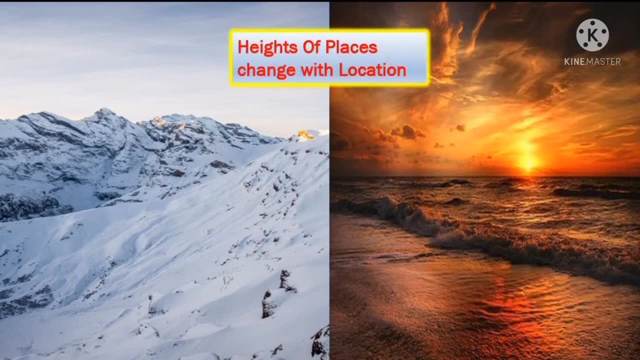 which are very common. So here we have a common view that people can either drop rock bottom or skyrocket with time, and also differ from country to country. Moreover, friends, not every place on earth is at the same altitude. The heights of different places change with each location And the value of assets like 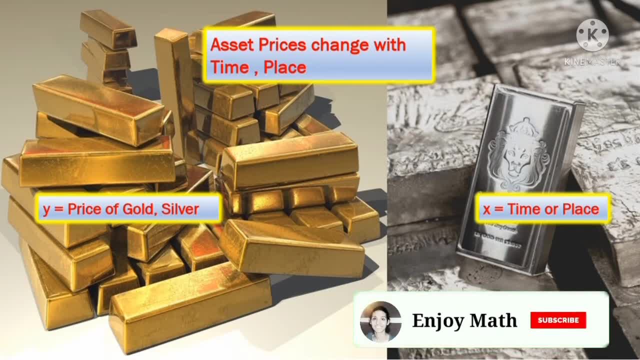 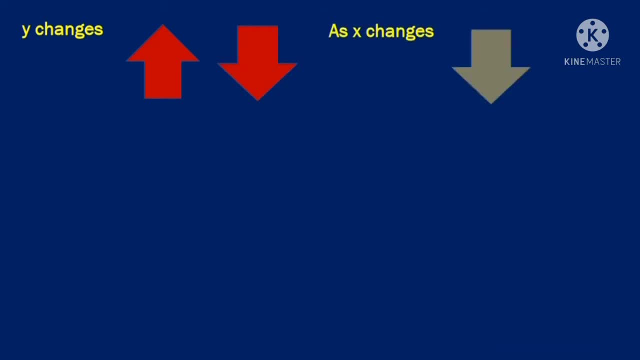 gold and silver fluctuate every day and also differ from country to country. y that changes its value whenever the value of another quantity, x, changes. So we can say that y is dependent on x or, broadly speaking, we can say that y is a function of x, which is usually. 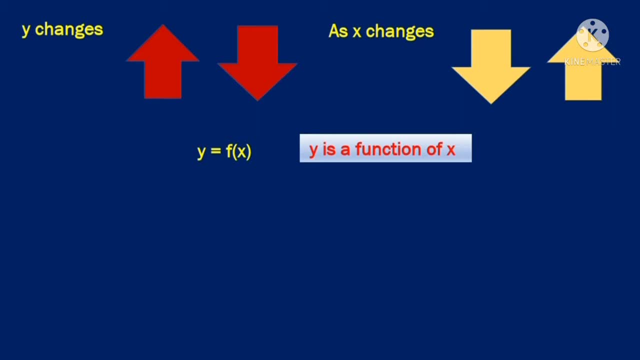 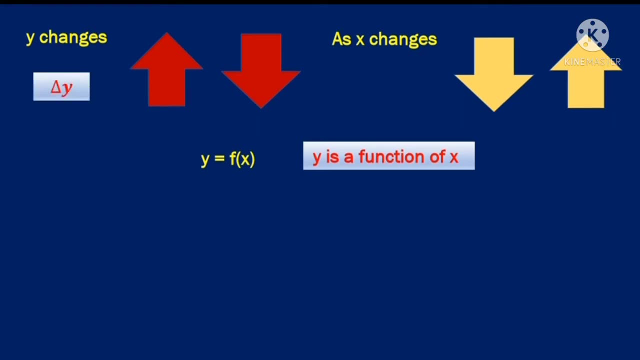 denoted as y equal to f of x. Also, friends, this change in y that we are talking about is usually denoted by delta y, which is nothing but the small triangle followed by y. So, definitely, the change in x will be denoted by delta x. Hence, the rate of change of y with respect to x is nothing but. 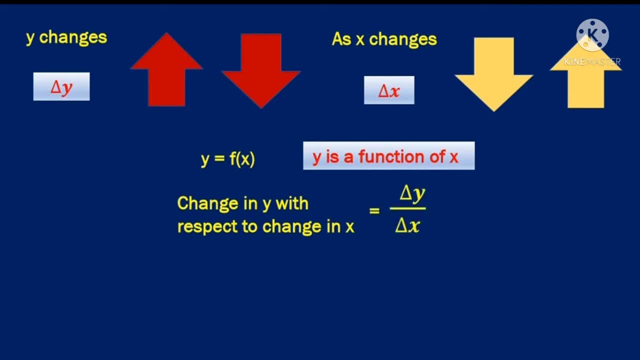 delta y upon delta x. Now, friends, here is an important point to ponder. When the change in x or delta x is very small, or tending to zero, then what happens? What happens to the value of delta y? Well, let's see this with an example. Let's suppose that a 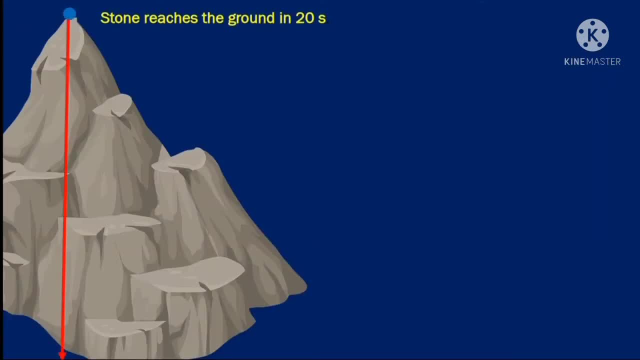 small stone is thrown from a hill and it reaches the ground in, say, 20 seconds. If y is the distance traveled by the stone, then, friends, using basic physics laws, we will get this equation that y equal to 4.9 t square, which connects the distance y with the time t. So definitely, as you can see. 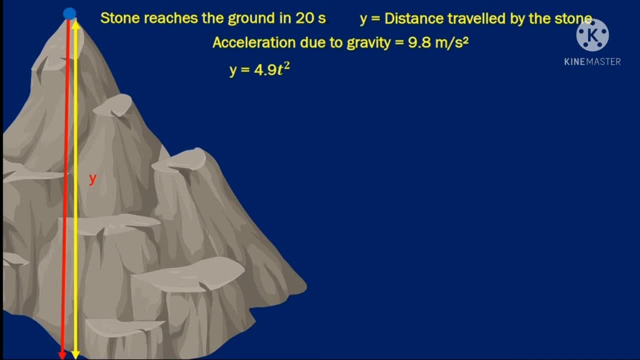 here y is the distance traveled by the stone. So let's suppose that y is the distance traveled by the stone. So let's suppose that y is the distance traveled by the stone. So let's suppose that y is dependent on t, So we can say that y is a function of t. So putting time as 20 seconds. 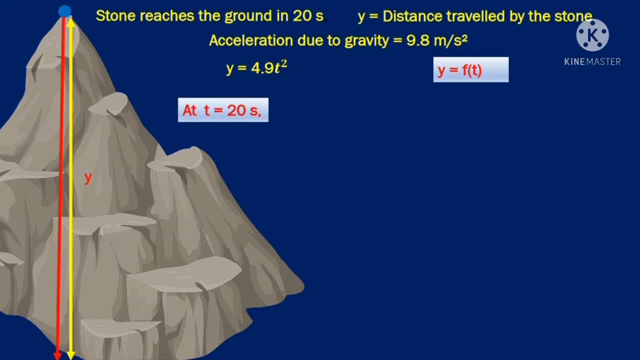 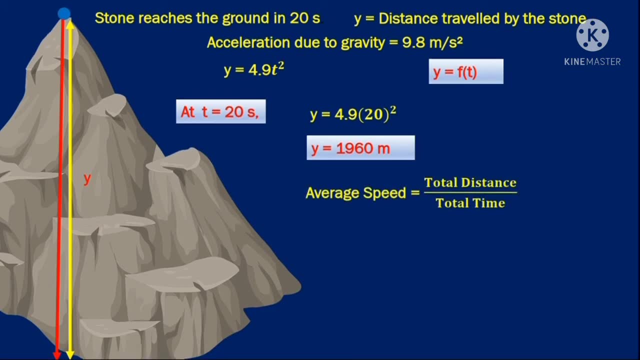 in the formula, we will easily get the distance traveled by the stone to be 1916 meters. So, friends, let's go ahead and also calculate the average speed of the stone, which is nothing but total distance divided by the total time. So, substituting the values, we get the average speed to be 98. 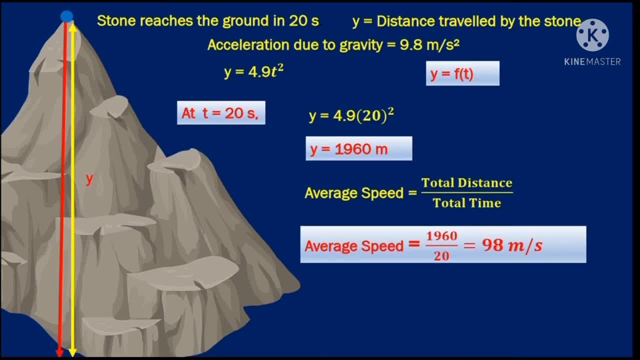 meters per second. Now, friends, all this is something that we already know. The big question is this: What is the speed of the stone at any particular instant, say at around 11 seconds? Will it be the same as the average speed of the stone? Well, it won't be, because there is acceleration. 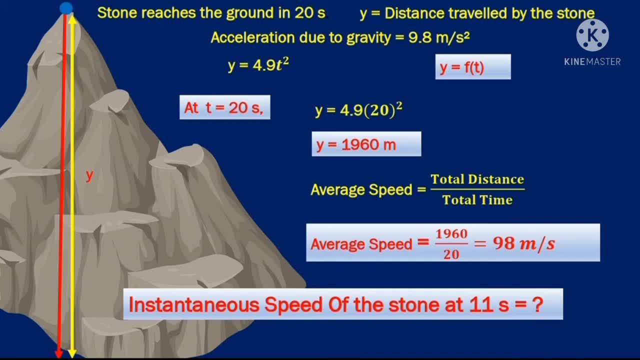 due to gravity, and hence the speed of the stone will be changing every second. So let's see how to find the instantaneous speed of the stone. So let's see how to find the instantaneous speed of the stone. So, friends, using the equation y equal to 4.9 t square, let's start filling this table. 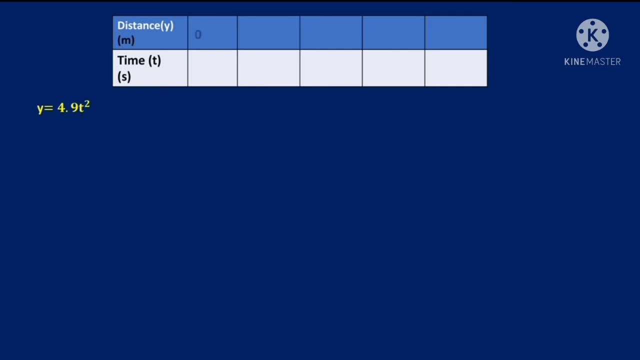 of distance and time. So, at t equal to 0, obviously the distance, y will be 0.. Now, at t equal to 11 seconds, for which we want the instantaneous speed, this is going to be y's value. Now, friends, let's take a time close to 11 seconds, say 11.1.. So the distance traveled by the stone will be 1916 meters. 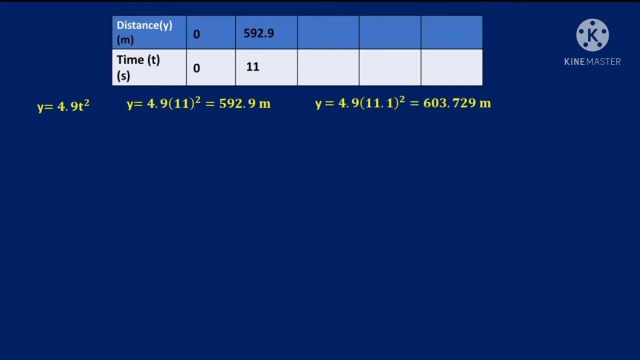 So the speed of the stone at 11.1 seconds is going to be 603.729 meters. Hence we can easily calculate the speed in the time interval 11 to 11.1 seconds as delta y upon delta t, which is nothing but these calculations, which gives us the speed to be 108.29 meters per second. 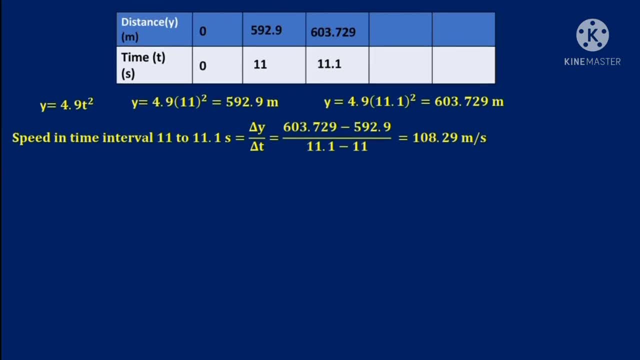 Now, friends, let's take another time interval which is even closer to 11, say 11.01.. And this is the distance that will be traveled by the stone at 11.01 seconds. Similarly, we can use the speed formula to calculate the speed in the time interval from 11 to 11.01 seconds, to be this. 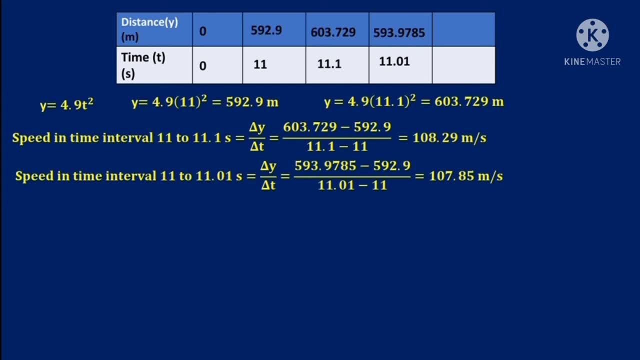 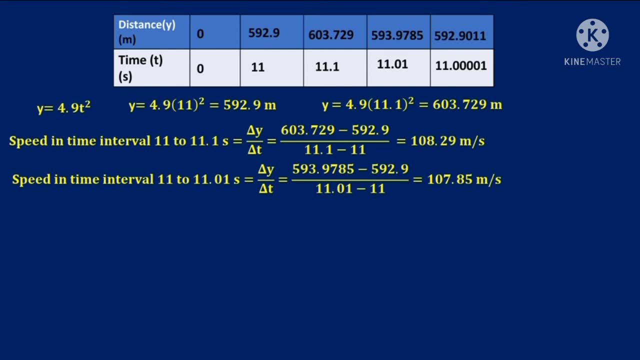 value. Now shall we go a step further, friends. Let's take the time interval to be 11.0001 seconds, and this is the distance y that will be traveled by the stone. Now did you observe that this time interval is closer to 11 than the previous two values that we took? So the delta t here will: 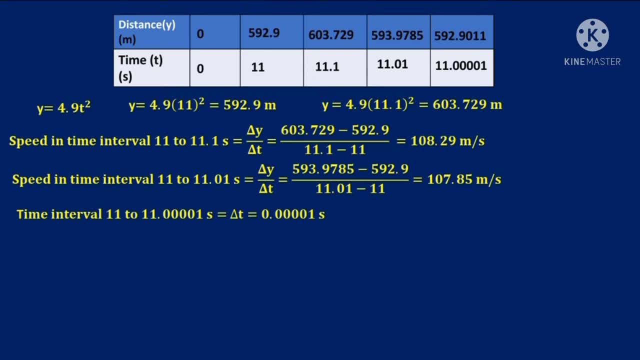 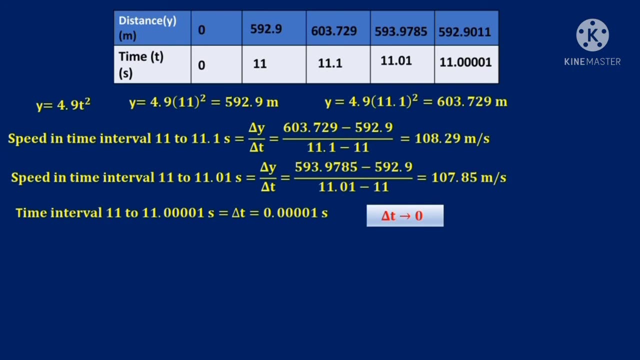 be 0.0001 seconds. So we can say that the delta t value here is very, very close to 0 or is tending to 0, and this is how we denote it by delta t tends to 0.. So, friends, the speed in this time interval. 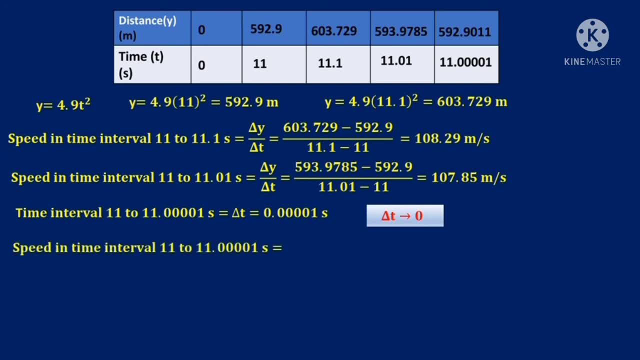 11 to 11.0001 seconds will be 0.0001 seconds, So we can say that the delta t value here is very, very close to 0.. So, friends, the speed in this time interval, 11 to 11.01 seconds, will be delta y by. 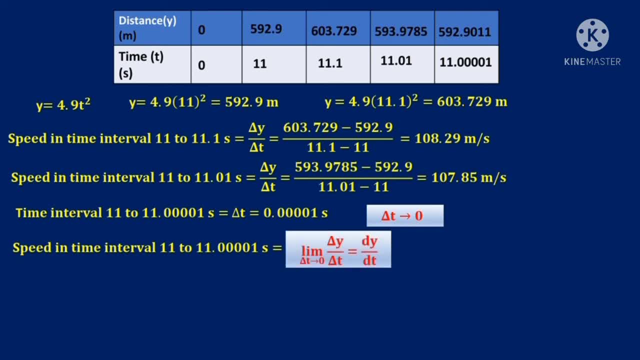 delta t. but, friends, the limit is that delta t is tending to 0 and it is at this stage that it transforms into dy by dt, which is also known as the derivative of y with respect to t. So, friends, calculating the speed in this time interval using the formula, we get the answer to be 110 meters per. 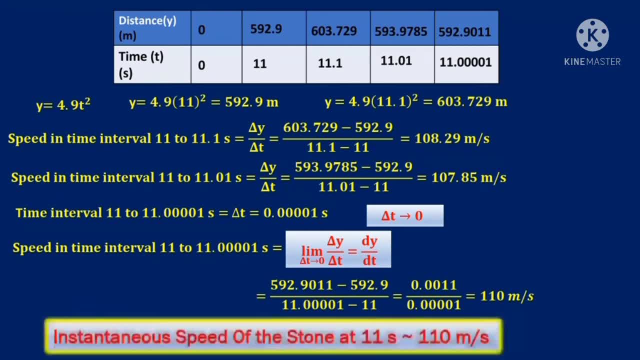 second. That means the instantaneous speed of the stone at 11 seconds is 0.0001 seconds. So, friends, this is the importance of differentiation. It helps us to calculate the change in y when the change in x is very, very less or tending to 0.. So, friends, let's now give the formal definition.